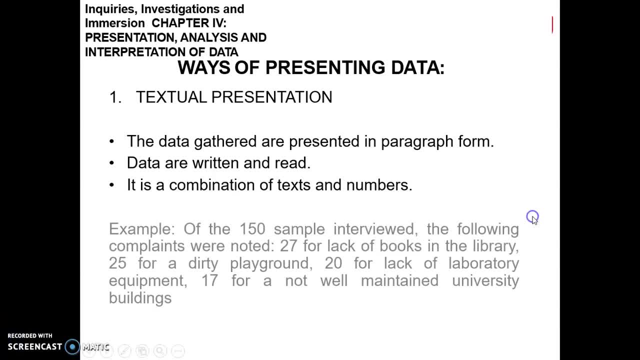 numbers. So an example is this one Of the 150 samples interviewed. the following complaints were noted: 27 for lack of books in the library, 25 for a dirty playground, 20 for lack of laboratory equipment, 17 for not well-maintained university buildings. 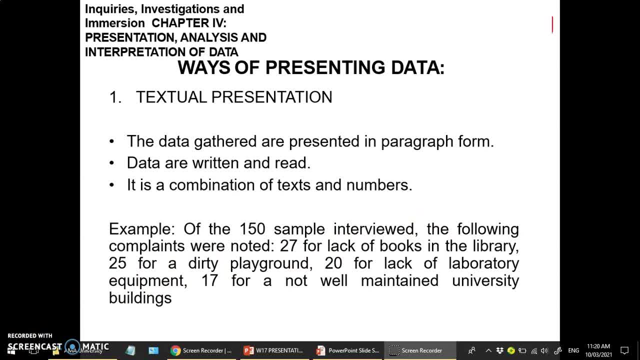 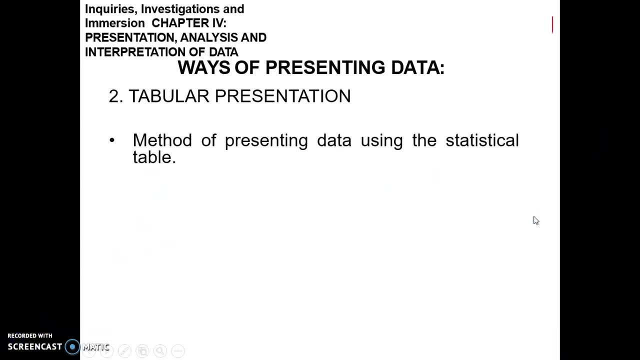 So this is an example of textual presentation of data. So it is in a paragraph form and it is just written and being read, and it is a combination of text and numbers. So let us move now to the tabular presentation. In tabular presentation, it is a method of presenting data using the statistical table. 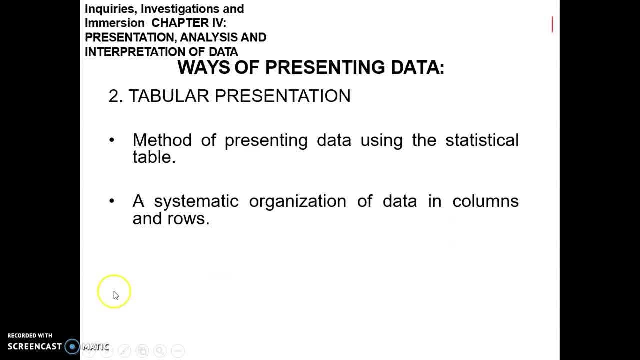 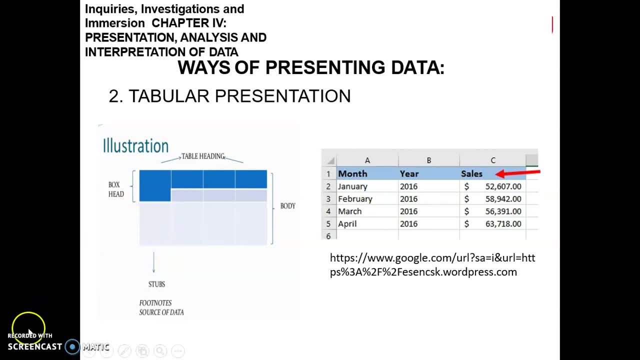 It is a systematic organization of data in columns and rows, So we can look at the graphics of the table and we can look at the tables and we can have more detail with the visual strategies using a tabular presentation. So here in the view, may we see this download: 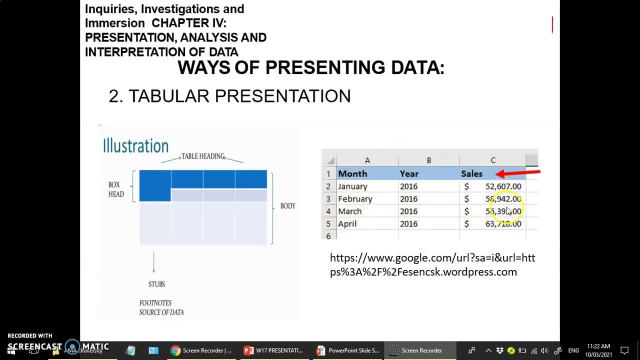 First, what we might see or will notice are tables. Next we reproduce the table Unidos. The tables also generate members as a parallel table. So we can see here, So we have each forward Duncan. This is the next past and we will view the data attestation of this table as our team overhand. 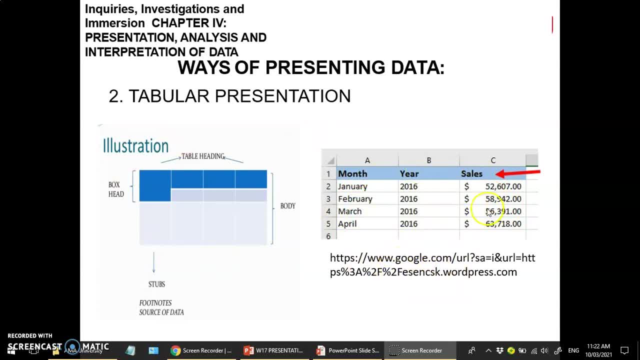 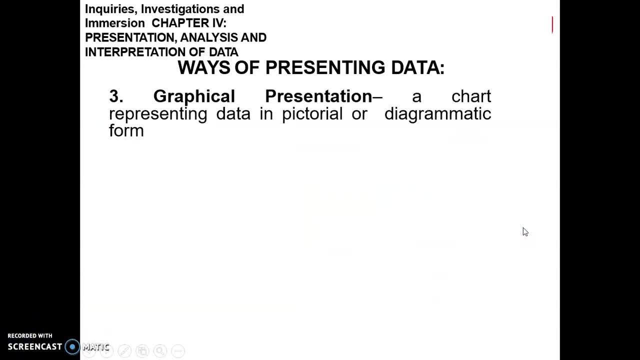 Now let us take a look at the minutes of today. watch for a moment. source of data. okay, so this is an example of a tabular data with columns and rows. so the third one is graphical presentation. it is a chart representing data in pictorial or 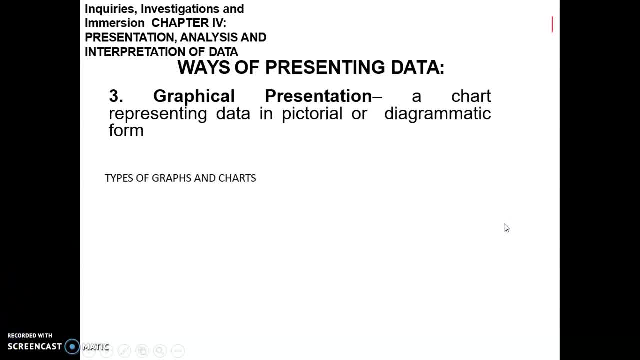 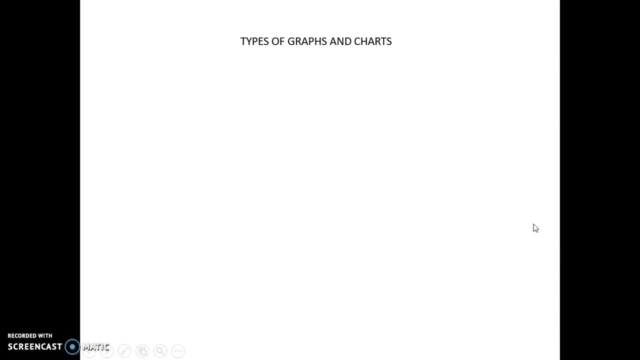 diagrammatic form. so we have different types of graphs and charts. so we have the bar graphs, linear graphs, pie graphs, pictograms, statistical maps and ratio charts. so to illustrate the types of graphs and charts, we have the bar graph. it looks like this: a linear graph or line graph a. 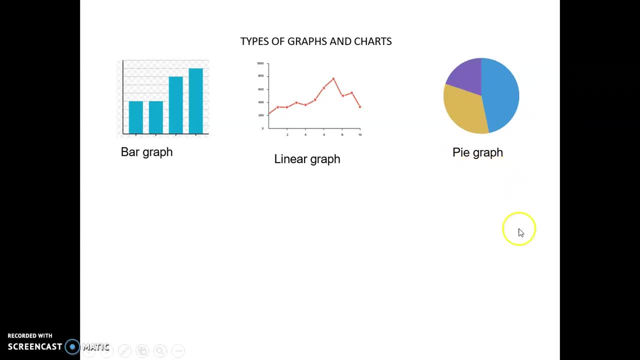 pie graph in circular form- pick the gram- with some pictures in it, a statistical map. so most of the time it is a map that includes some information like population, some harvest amount, something like that, and lastly a ratio chart. a ratio chart includes two different kind of data. so here we have two kinds of data: the green one and the darker one. so 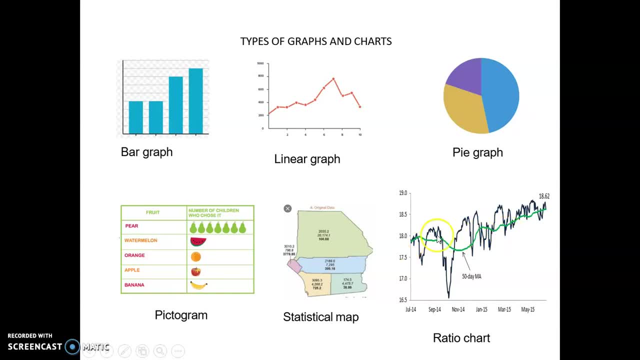 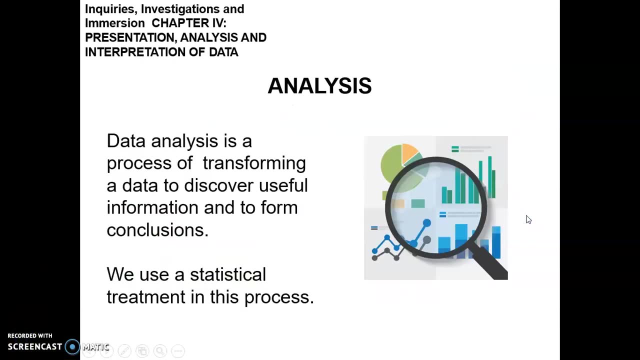 the purpose of ratio chart is to compare these two, these two data sets. so let us go now to the analysis of data. data analysis is a process of transforming a data to discover useful information and to form conclusions. we use a statistic, that we use a statistical treatment in this process, so to be able to analyze. 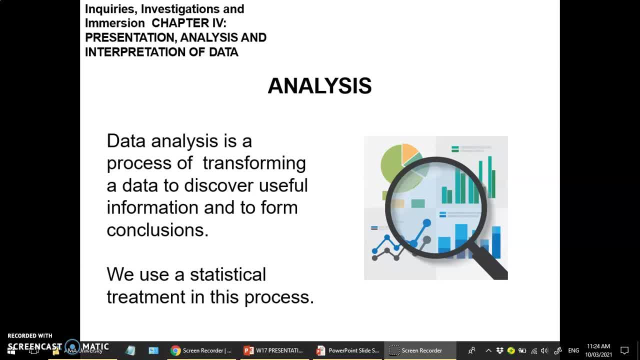 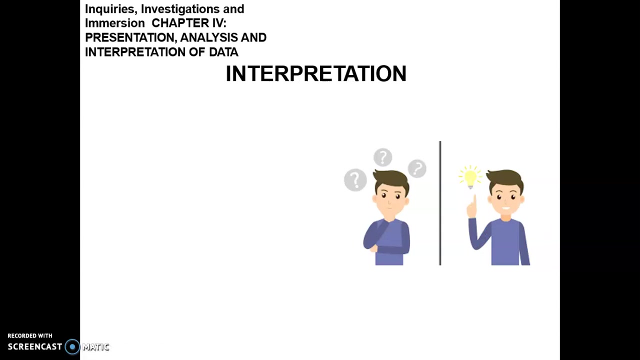 data. we use some statistical processes like central tendency, mean mode, median. also we can use some percentage or we can use some advanced physical treatment like t-test, p-test, analysis of variance and chi-square test. so in this part we use the statistical treatment that we studied last week and finally we have the interpretation. 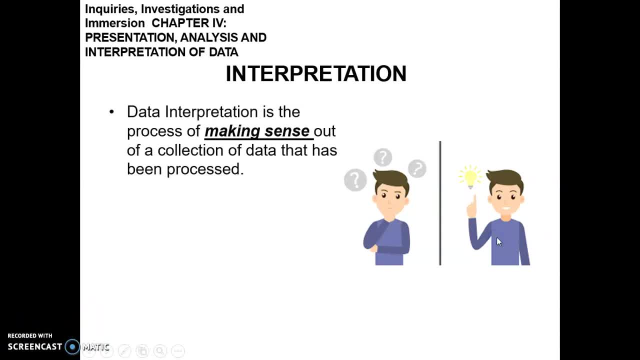 in data interpretation. it is the process of making sense out of a collection of data that has been processed. so, since we have this data that we collected, what do the results of the study mean? this part is perhaps the most critical aspect of research report, and this will constitute 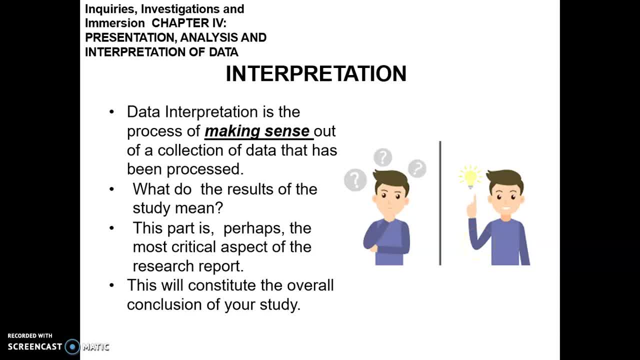 the overall conclusion of your study. so your study will rely on the interpretation of the gathered data. so that's the, that's the data supports or go against your hypothesis, something like that. so I'm hoping that that makes sense, because the interpretation of data is being done by the researcher, basing his conclusion on the gathered data. 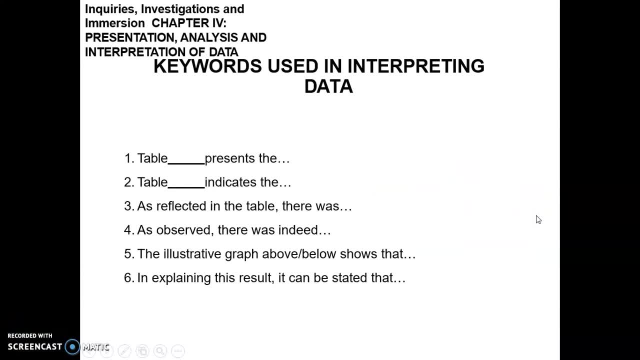 okay, so the keywords in interpreting data are as follows. so, for example, table blank presents the another is a table blank indicates law, so it also could be as reflected in the table. there was blank, something like that, as observed, there was indeed. the illustrative graph above or below shows that. 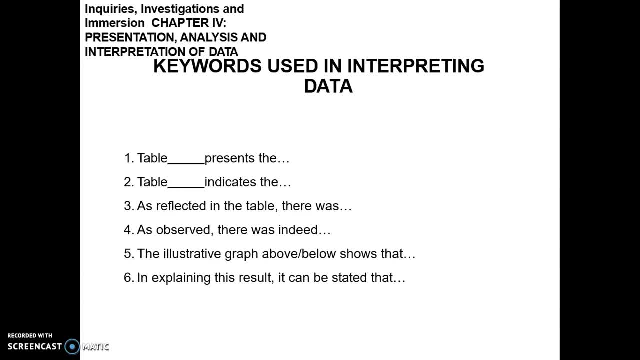 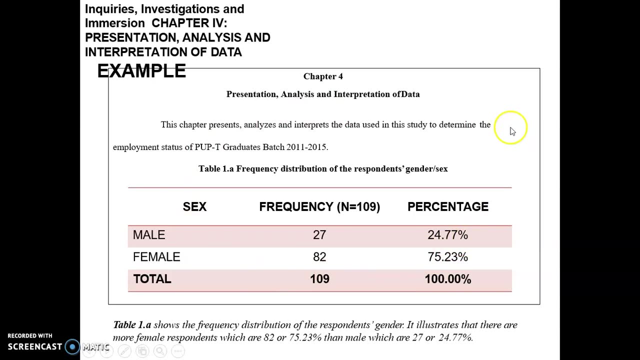 and it also can be in explaining this result. it can be stated that. so these are the keywords we use in interpreting data. so this is an example of a presentation, analysis and interpretation of data. so we can see here that the interpretation is in tabular form. we have a table, so we have sex and frequency. 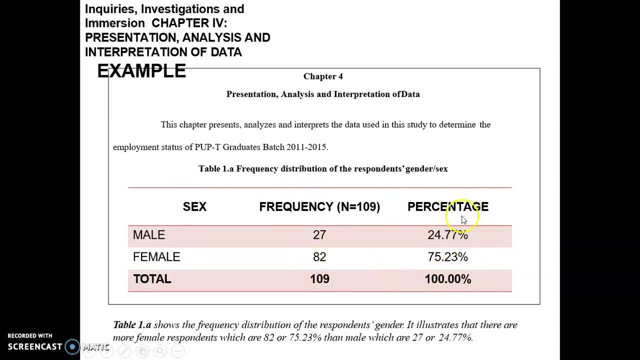 also the analysis is in terms of percentage. so we just get the percentage of male versus female here and the interpretation is here below. so it shows that the frequency distribution of respondents- gender- it- illustrates that we are, that there are more female respondents, which are 82 or 75.23 percent, than male, which are 27 or 24.77 percent. so this is. 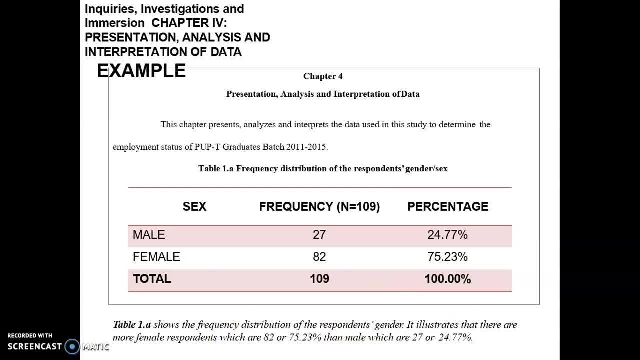 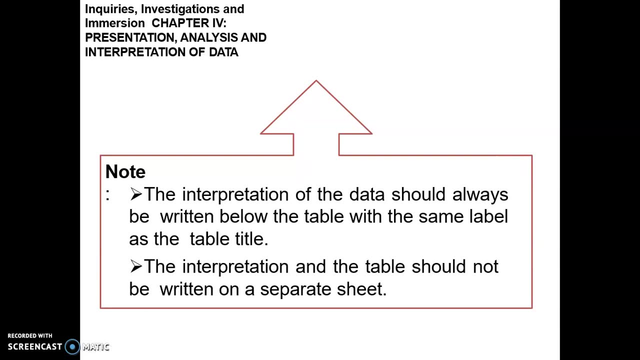 an example of combination of presentation, analysis and interpretation of data. okay, so i'm hoping that this is easy enough for us. so we have some notes here. so the interpretation of data should always be written below the table with the same label as the table title. okay, so the interpretation is always below the table. 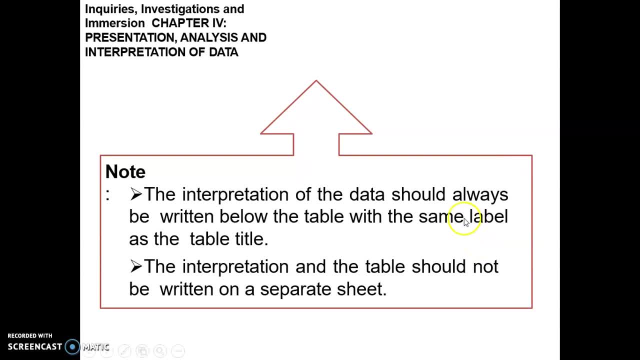 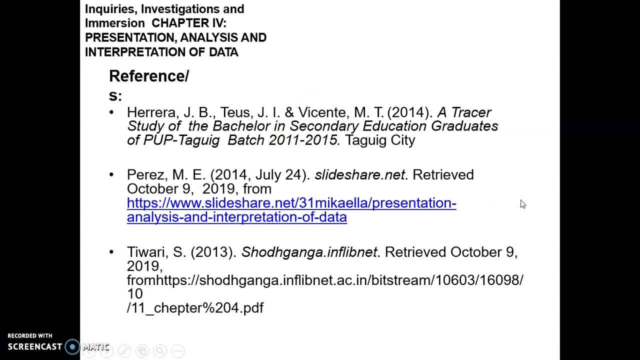 it that should not go above the table, only below, okay. and the interpretation and table should not be written on a separate sheet. so as much as possible we write them or type them in the same sheet so that the reader can understand the table clearly and immediately. so that is all for our presentation. analysis. interpretation of 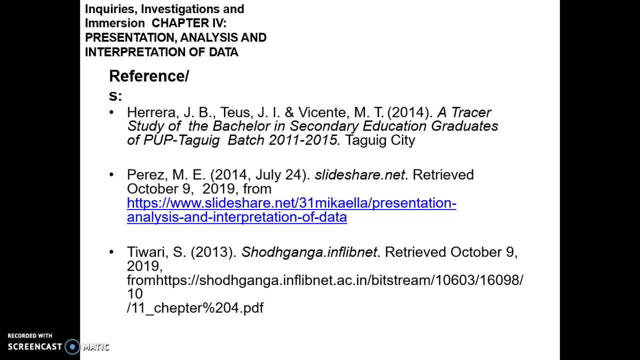 data lecture. so i'm hoping that, uh, everything i said makes sense to you and thank you for listening.